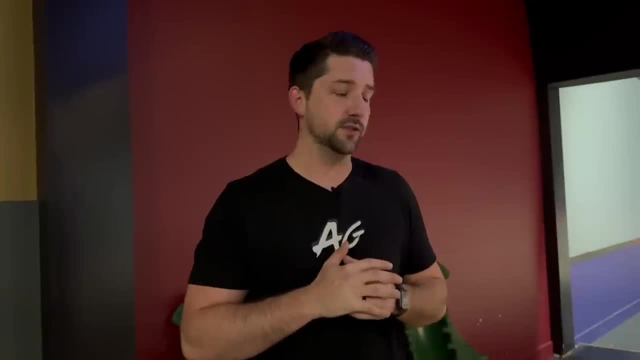 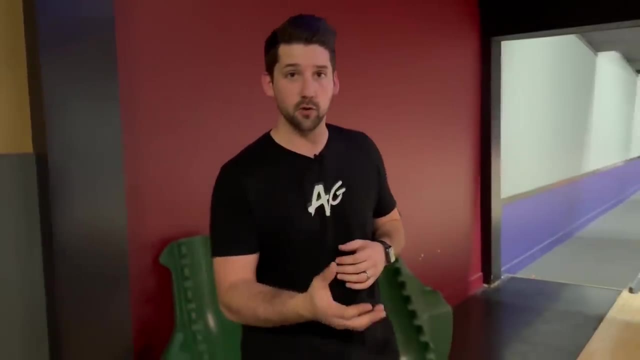 What's up guys? welcome back to the channel. So today we're going to be doing a how-to video on how to hook the bowling ball. I've had a lot of people in my comments requesting that I show or explain how I hook the bowling ball, and so we're going to get into that today. I'm going to try to. 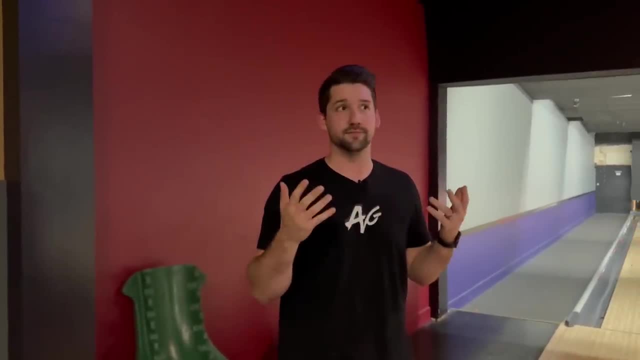 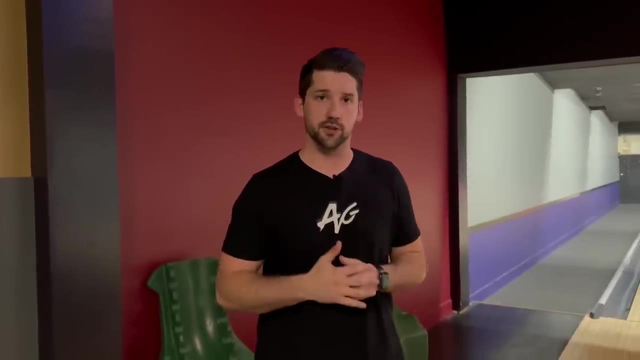 explain it the simplest way possible, the way that I was taught, like 17 years ago now. Obviously it's evolved since then, but the basics of how to hook a bowling ball, the proper way is what I'm going to show you today. If you're new to bowling, naturally to hook the bowling ball, you think. 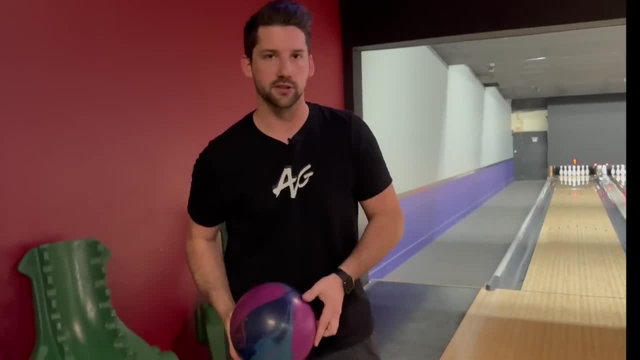 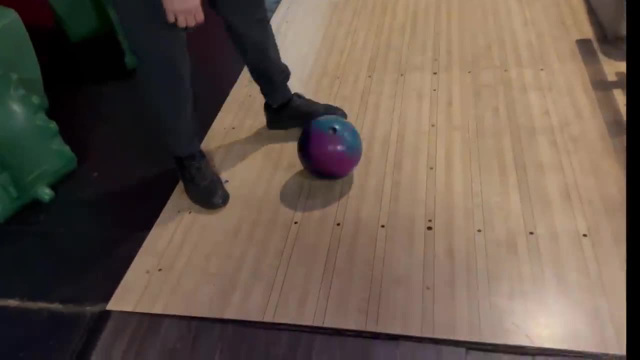 you have to spin over the top of the ball to get the ball to rotate. So you end up spinning your entire wrist over the top of the ball to cause the rotation. like a top spin like this, When really you want to think of it as like a football, Like if you're underhanding a spiral football. 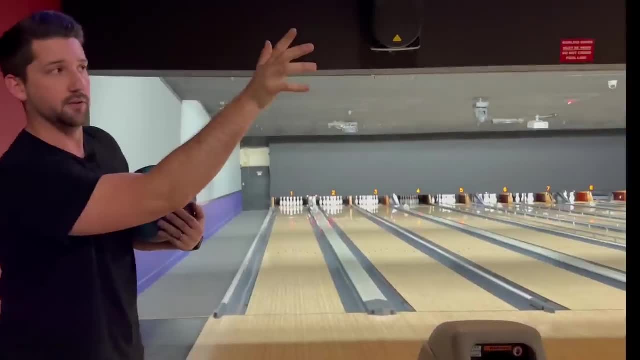 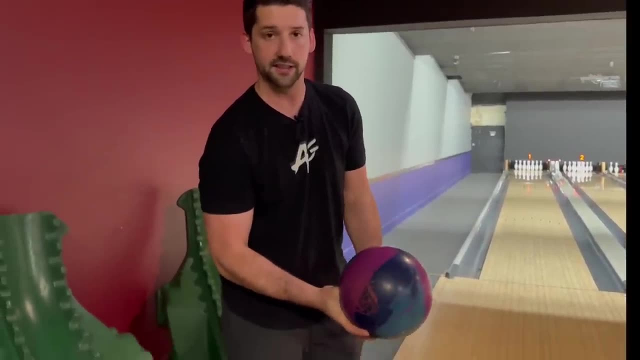 you're going to pull the football back and you're going to release it like a spiral and your thumb is going to be pointed to the sky. It's the exact same thing with a bowling ball. You want your hand to be directly behind the bowling ball at the release, so when you're coming through, it's behind. 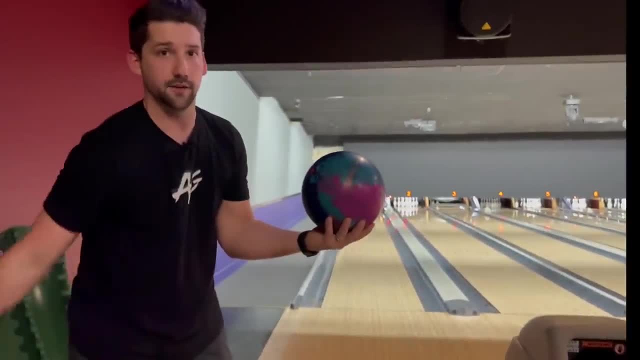 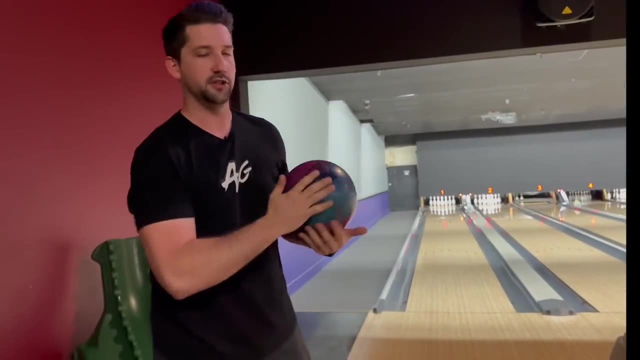 the ball and then you're spinning like a, like a football, with a thumb to the sky. So it's just a one fluid motion: spin, thumb to the sky. I'll show you more closely at the foul line. So, like I said, when you're starting out typically and you're going to release and you're a brand new, 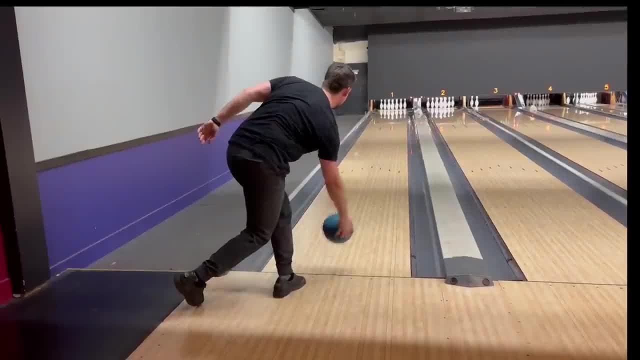 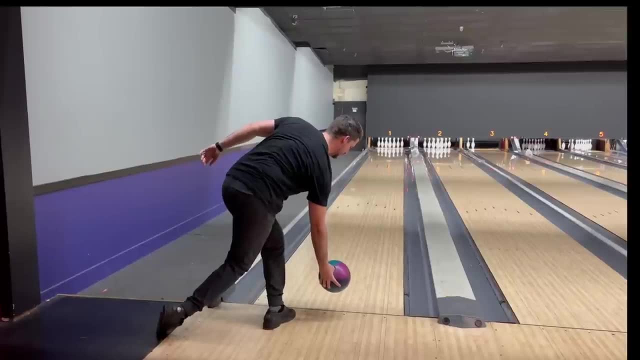 bowler, you want to come over the top of the ball. That's your tendency, because you think, oh, I want to hook the ball, so I must have to come over the top of it, When really you want, at release your ball, to be directly behind the ball and just rolling it forward. 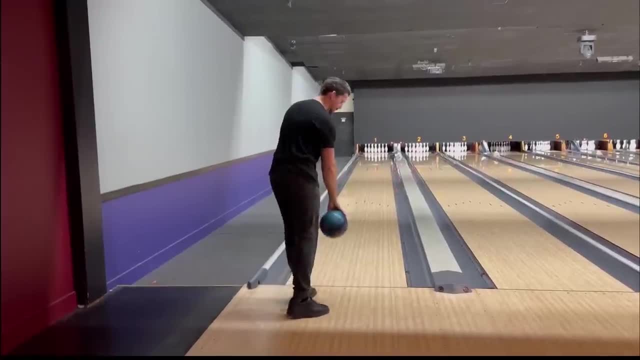 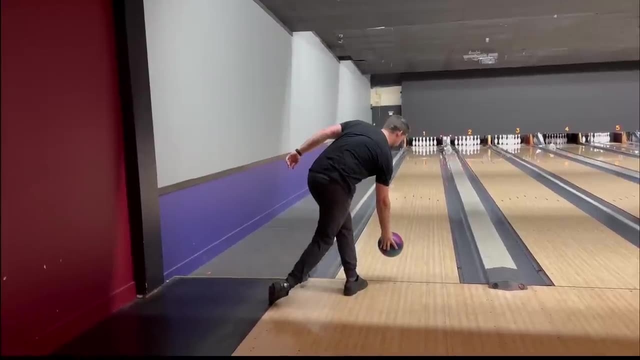 This creates what's called forward roll. So yeah, like I said, if I were, if I were just starting again, I would say the main thing to work on is staying directly behind the ball at release. Take a video of yourself staying behind the ball at release and rotating almost as if you're. 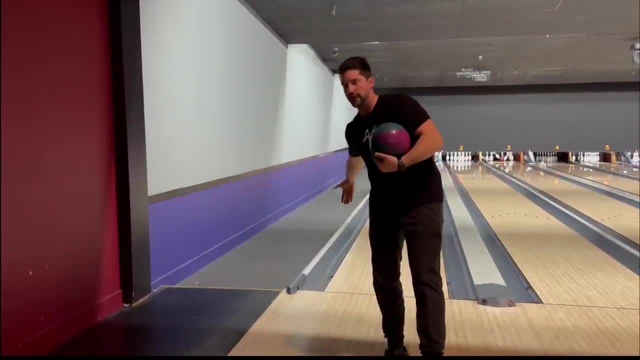 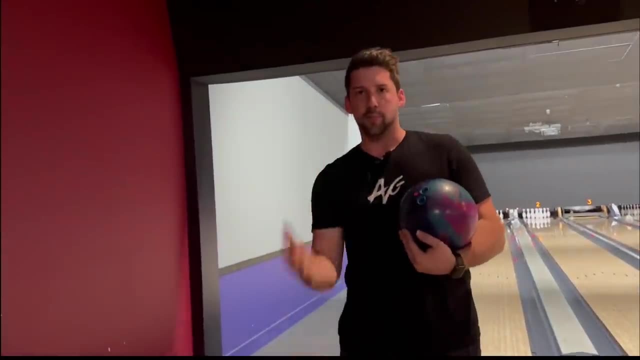 shaking somebody's hand, Pulling the ball back straight, and then you're coming through, you're shaking somebody's hand at release thumb into the sky. That will get you the basics of getting proper rotation on the ball and then from there it's just developing the wrist strength to 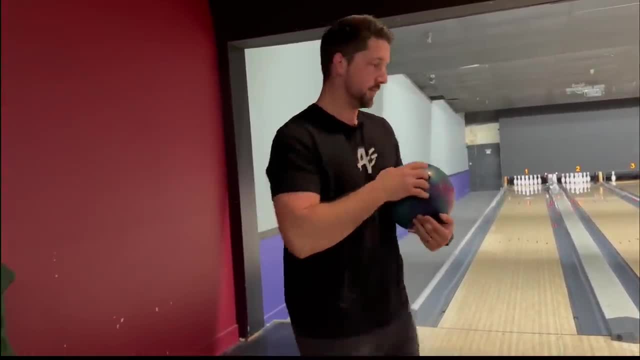 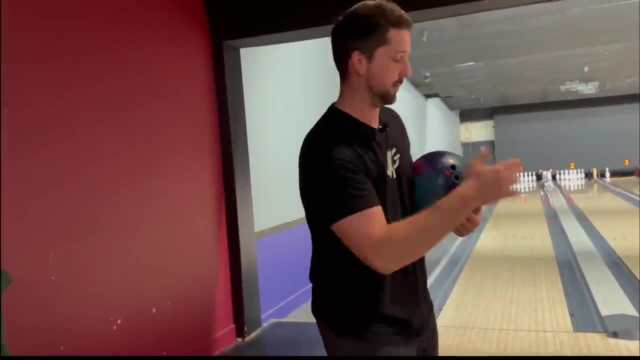 be able to create more of like a yo-yo snap at the bottom, Which all the pros do, You'll see, they load up and they snap at the bottom, kind of like a yo-yo. You know, hinges and unhinges at the bottom. 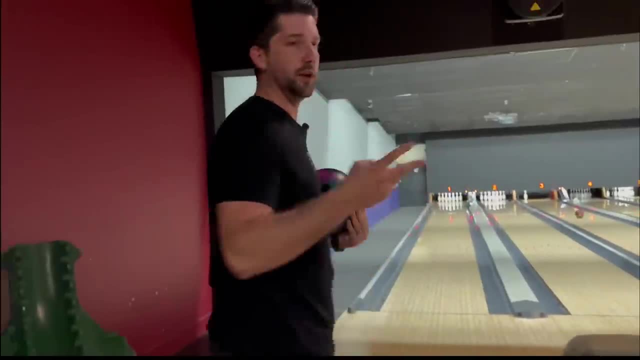 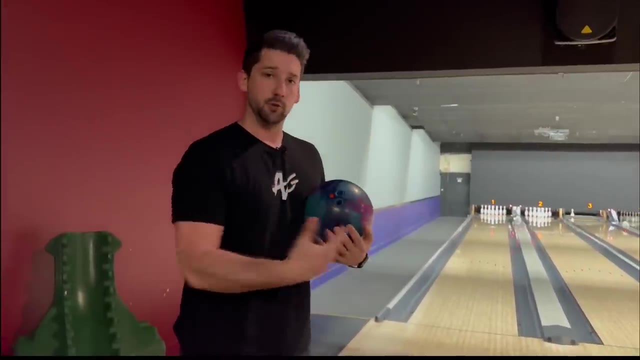 So here's an example. Now, this is one of my two releases that I do, because, as you start bowling more competitively on challenging sport patterns, you want to be able to switch up your rotation a little bit. So this is my stance and I'm going to show you how I do it. I'm going to show you how I. 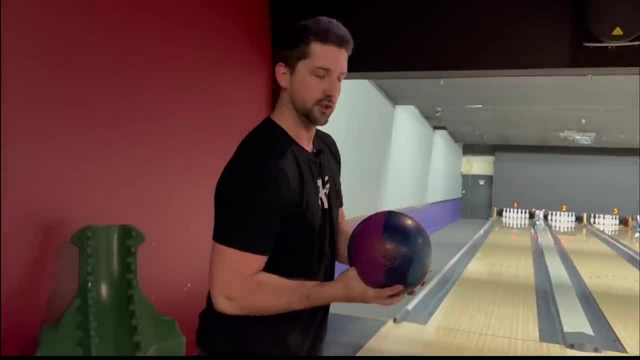 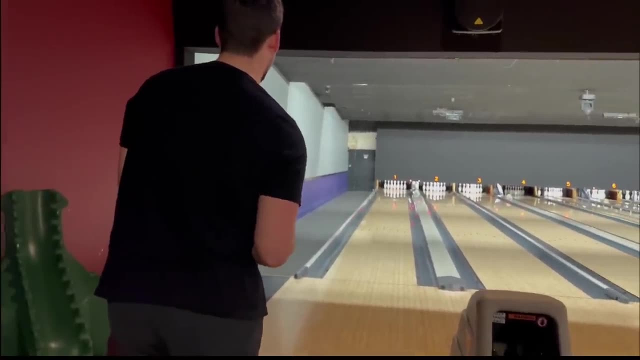 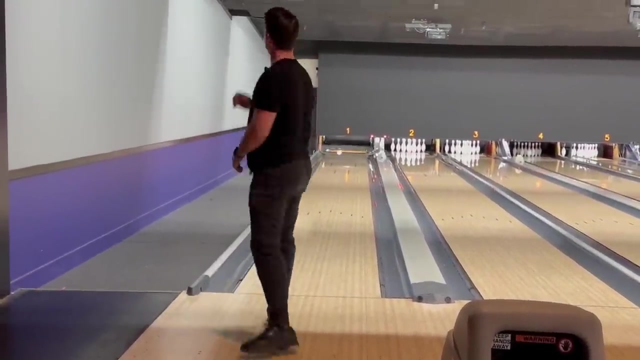 do it. I'm just going to take a standard neutral position that I call just standard forward roll, just directly behind the ball. It's not going to create an insane amount of rotation, but it'll be enough for typically house shots and shorter patterns. So you can see my ball roll was going really forward. I'm not going to be moving too much. 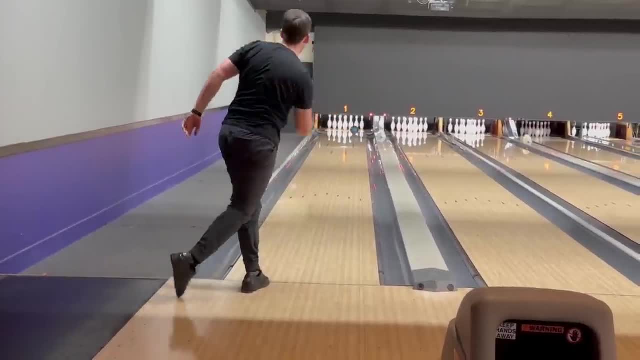 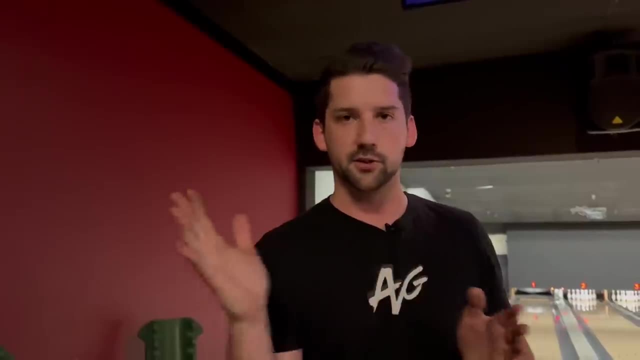 I'm going to be moving a little bit more to the side and then I'm going to go straight forward and then I'm going to go back to the starting position. So that's just a little bit more of an really forward. and had a very smooth, controllable motion down lane wasn't too snappy, didn't hook. 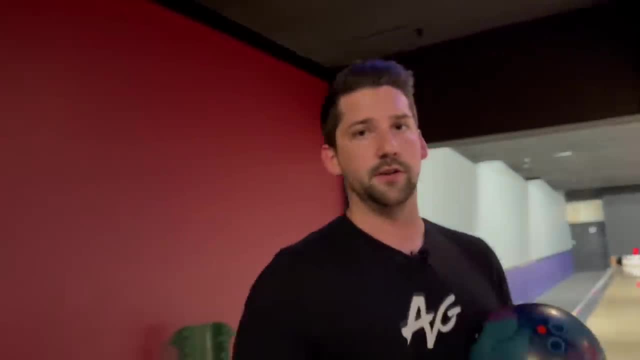 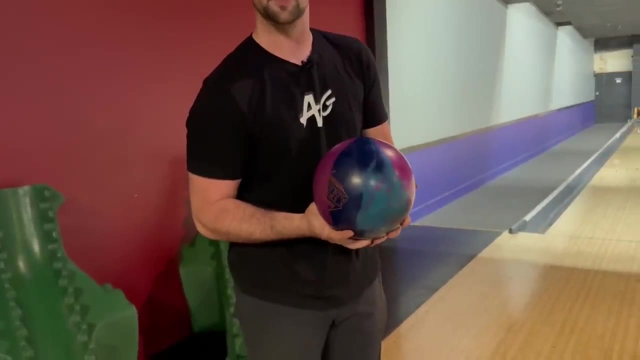 too early. So now for the more advanced bowlers. if you're looking to try and create more rotation on the ball, typically what I would like to do is go from your standard neutral position of just being behind it and just rotate your wrist inside, which is what's called more of a loaded position. 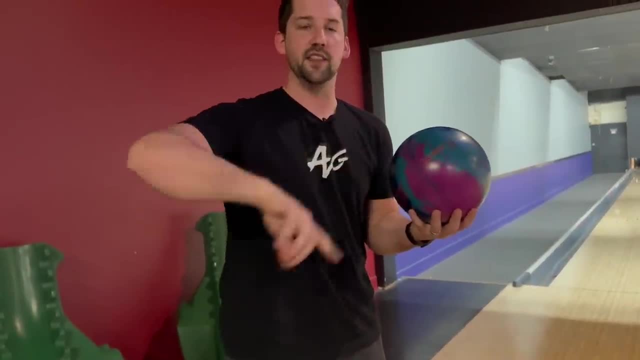 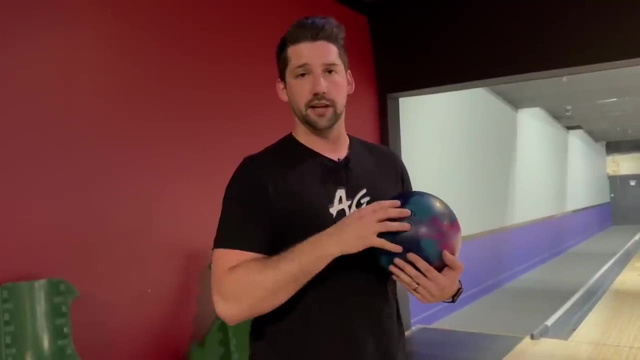 It's going to create it, so you're naturally going to start spinning the ball a lot heavier. It's going to create a lot more rotation, be good for longer patterns and when you need to slow the ball down and hook the lane a lot. So let me show you an example of that. So now I'm going to move. 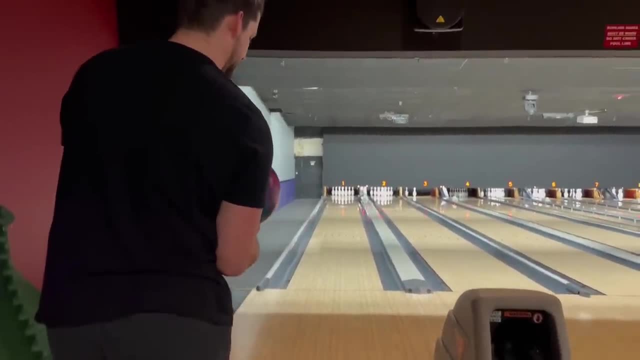 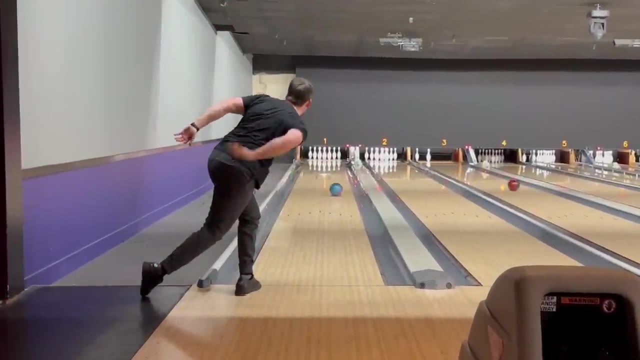 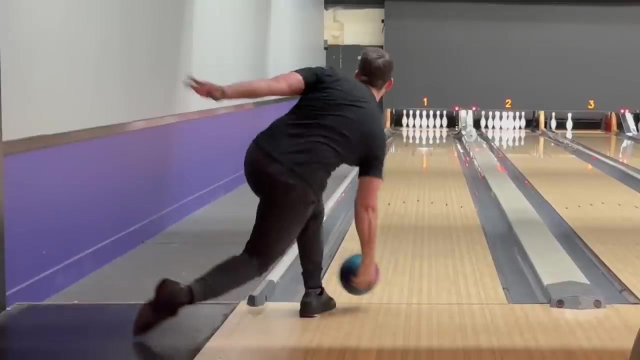 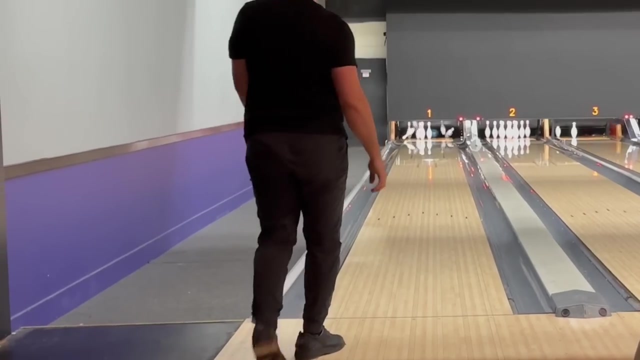 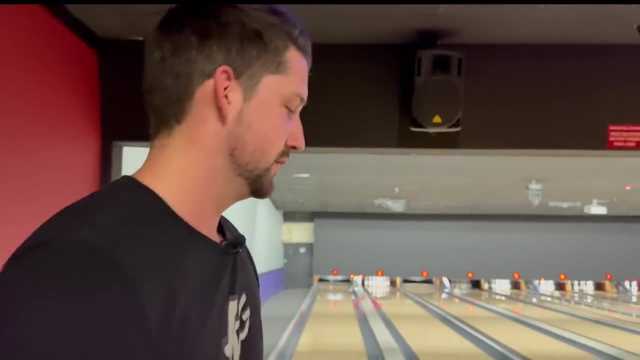 off my last shot. We're going to turn the wrist inside to the loaded position and we should get the ball to hook more. So that was a little wide of my target, but you can see it still made the turn harder. Let me do one more.